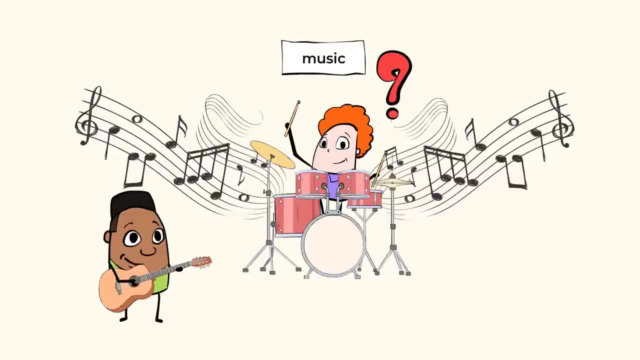 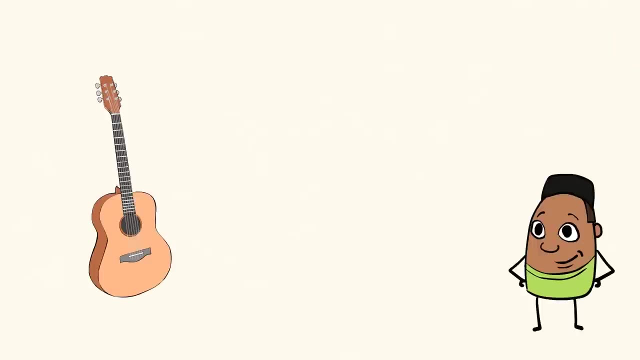 Huh, but how do those instruments create sound in the first place? What is going on when we hear sounds? Well, it's all about vibrations. What are vibrations, you might ask Rightly. so Well, let's take a closer look at that guitar to perhaps find an answer to our question. 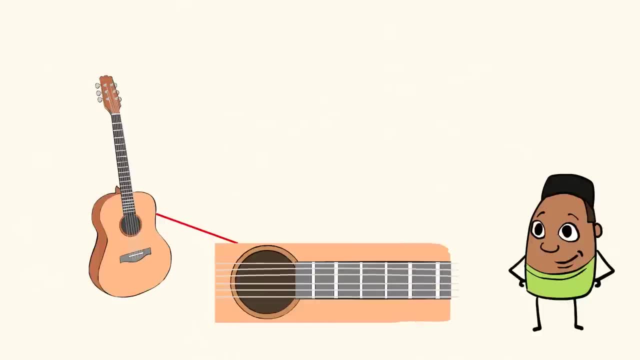 Now watch what happens when these guitar strings get plucked. Cool, Did you see that Those strings are moving back and forth really quickly, And that is vibrato Vibration. When an object moves back and forth quickly, it's vibrating. 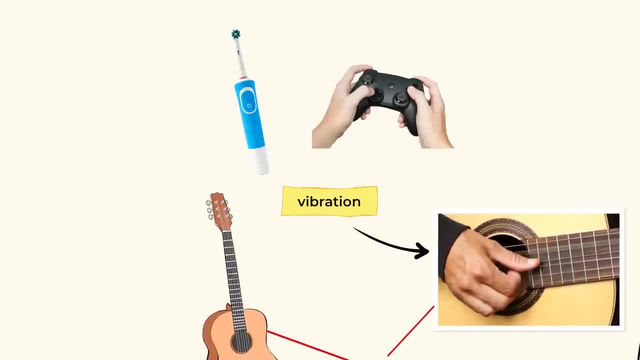 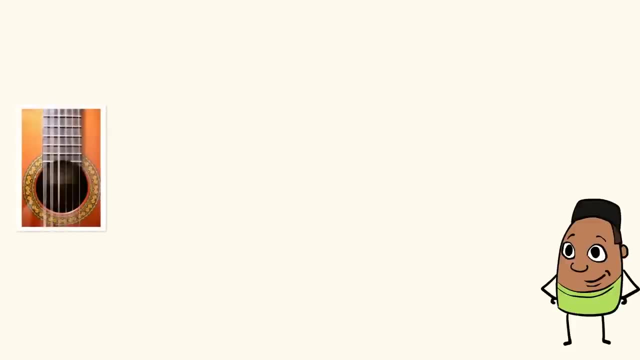 Kind of like your electric toothbrush or a video game controller. Wow, look how fast those strings are moving. Now, when the strings move back and forth, they also move tiny particles that are roaming freely in the air. This movement creates what is called a sound wave. 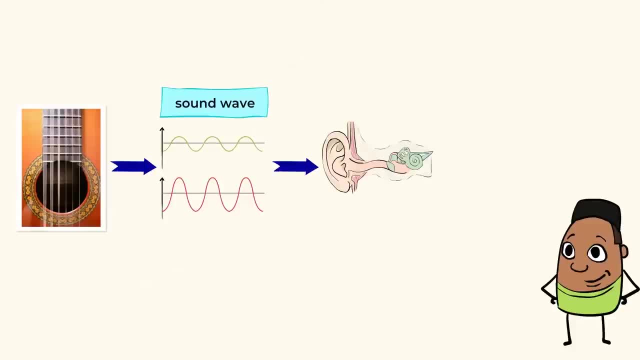 These waves travel through the air, and when they reach our ears, they cause a part of our ear called the eardrum to vibrate. And when the eardrum vibrates, it then sends sound signals to our brain And that's how we hear sounds. 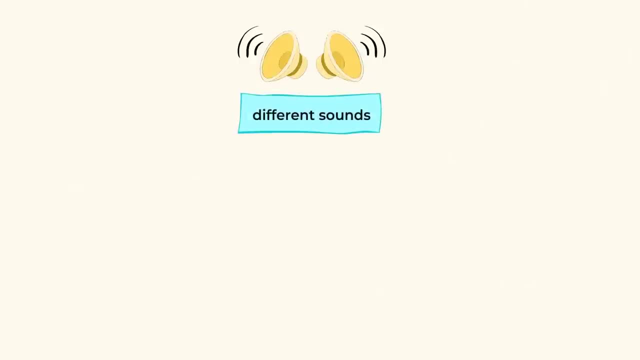 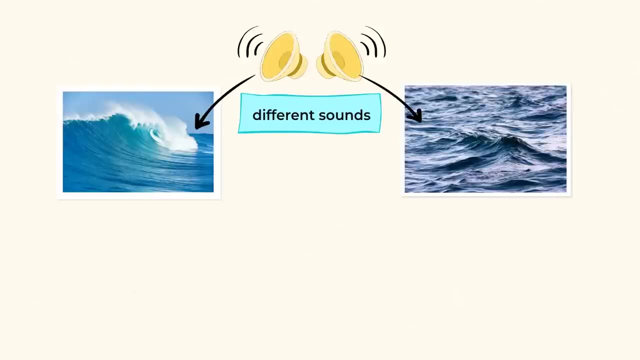 How cool is that There are all sorts of sounds and different sounds create different waves, Just like waves in the ocean. some waves are big and some are small. The bigger the wave, the louder the sound. If the guitar string is plucked very gently, 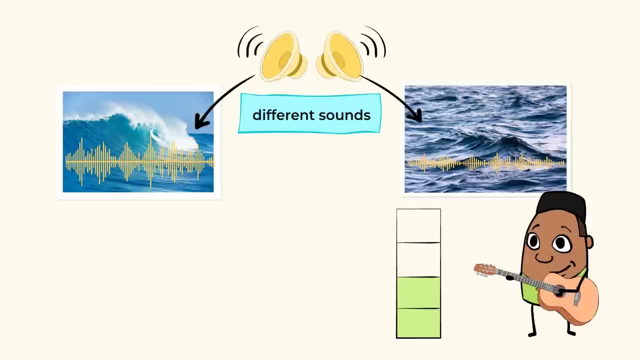 it'll create a quiet sound, But if it's plucked with more power, it'll create larger waves through the air and therefore a louder sound. Cool right Now. here's an investigation that I invite you to do on your own. 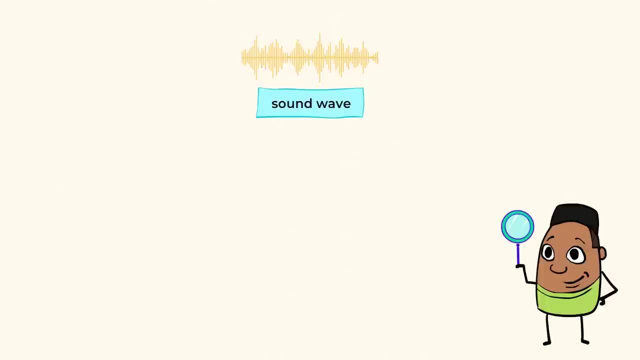 in order to learn more about sound waves. Here we go. All you have to do is gather up these materials: A small box and four to six, Six, rubber bands. Next, stretch the rubber bands over the box And now try to pluck the rubber bands, one at a time. 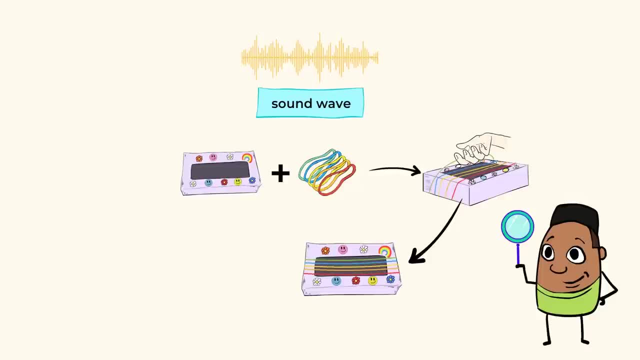 The rubber bands vibrate when you pluck them and you'll hear a sound. Try plucking some of them very softly. Well, how does that change the sound that you hear? What if you pluck a rubber band harder? Do you hear a louder sound? 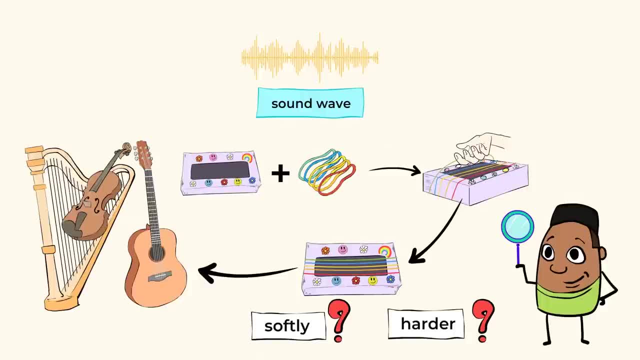 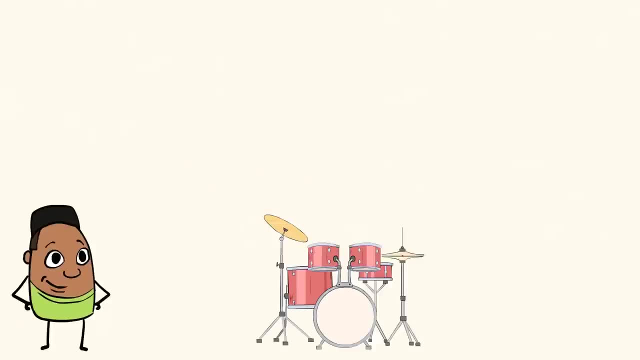 All instruments with strings work this way, but other instruments are great too for learning about how sound is produced. Let's look at one of my favorite: the drums. A drum has a thin layer called the drum skin stretched across the top of it. 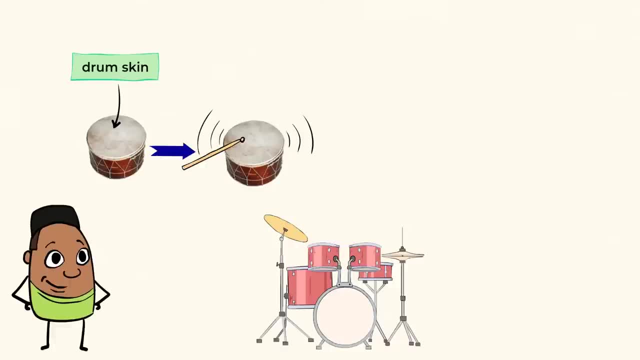 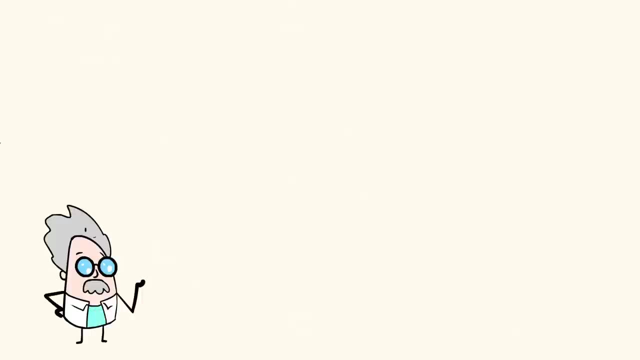 When you hit that with something like a drumstick, then the thin layer vibrates. The vibration travels through the air to our ears. Oh, have I got a cool trick up my sleeve? Watch what happens when some salt is poured on the drum. 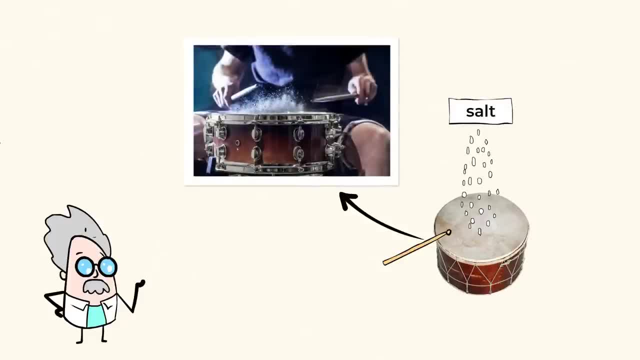 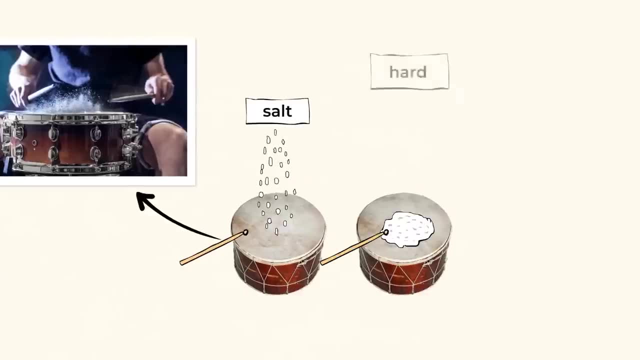 These salt crystals make it easier to see the vibration happening when we hit the drum. You can see them bounce up and down as the drum vibrates. If we hit the drum hard, they bounce higher. If we hit it gently, they bounce lower. 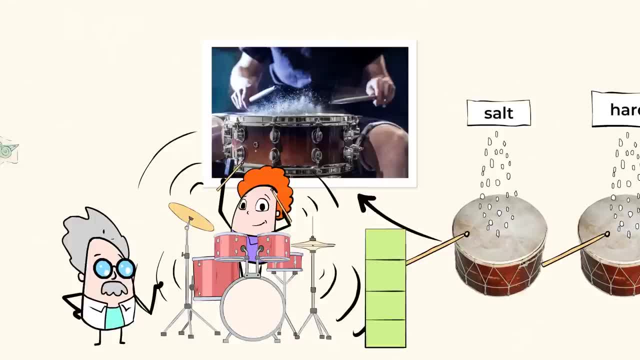 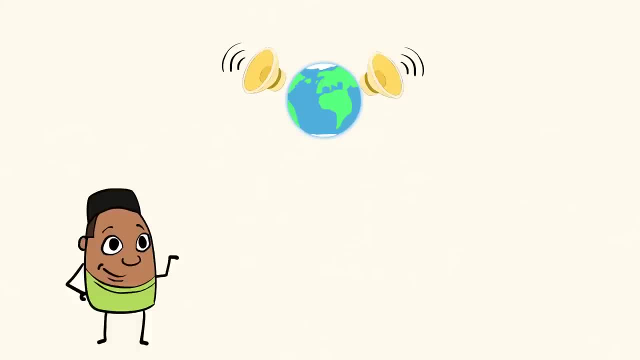 The harder you hit a drum, the louder the sound you will hear. So far today we've been quite musical, but there are so many different sounds in our world and different objects make different sounds. Some are really quiet. It sounds like a whisper. 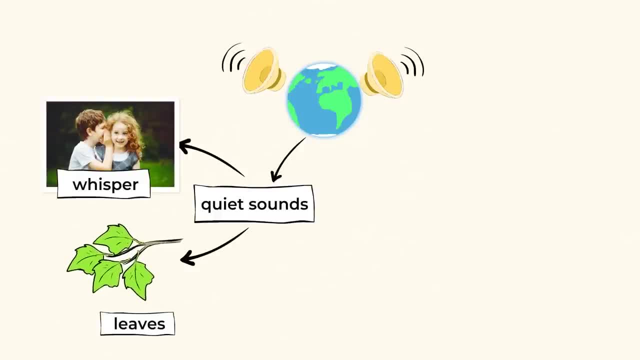 or leaves rustling in the wind. The leaves are only moving a little bit, so they create small vibrations. Ah, these sounds are quite soft and relaxing, aren't they? Ooh, but there are also loud sounds like a horn honking or a whistle blowing. 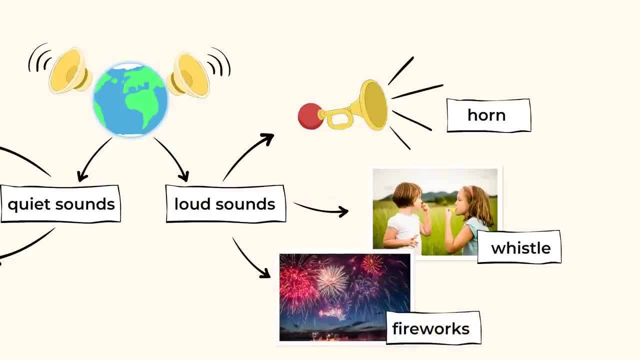 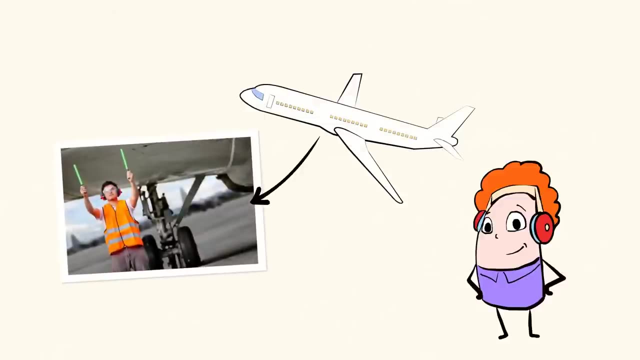 Oh wow, you might need some earplugs for those sounds. The sound waves that are made by fireworks are also very big, which makes the sound that we hear very loud. Look at Eric. He obviously knows the plane's engines will be very loud. 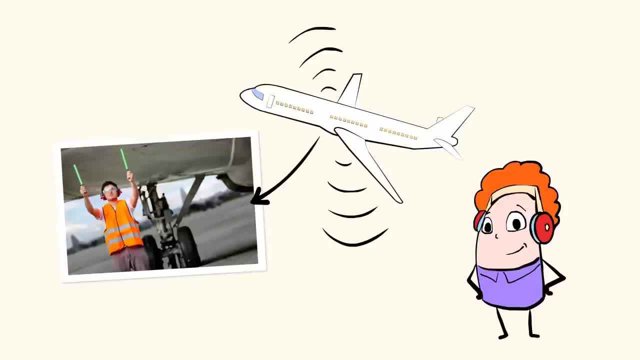 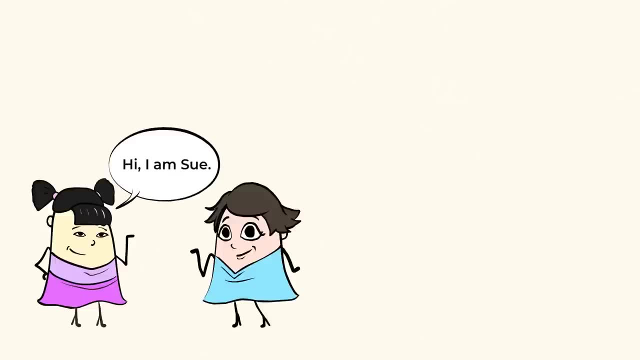 And that's why he has headphones on to protect his ears from the extremely loud sounds. And we can also create sounds with our bodies too. Think about how you might tell someone your name. You might say it out loud. right, Try it out. 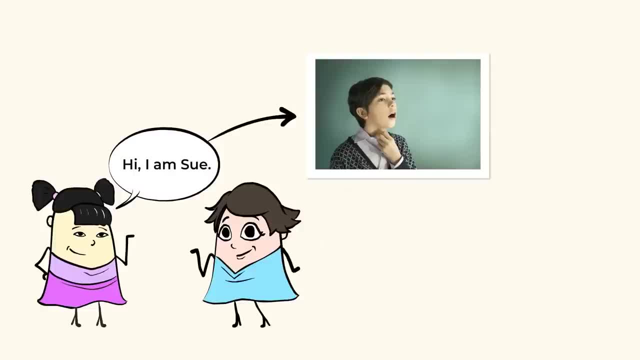 try this: Say your name really slowly and put your hand gently on your throat. You'll feel a little buzzing. That buzzing is created by your vocal cords vibrating in your throat. Your vocal cords are like little rubber bands that vibrate to make the sound of our voice. It's kind of like